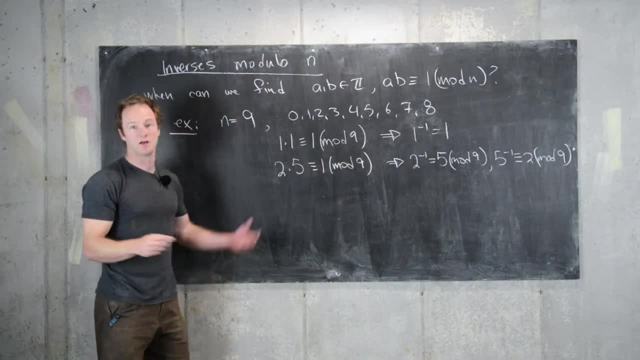 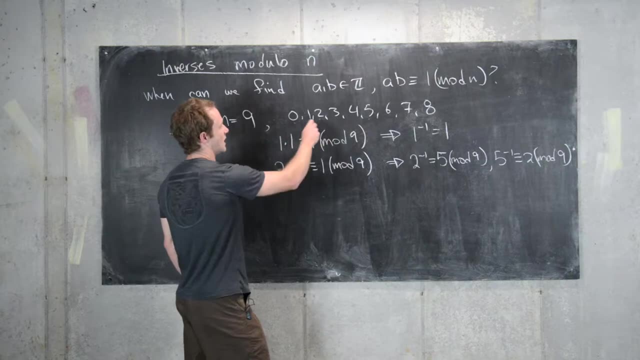 Obviously, 0 doesn't have an inverse modulo n for any n, because 0 times anything is 0. You can't ever get to 1.. So let's look at some others. So we've taken care of 0,, 1,, 2.. 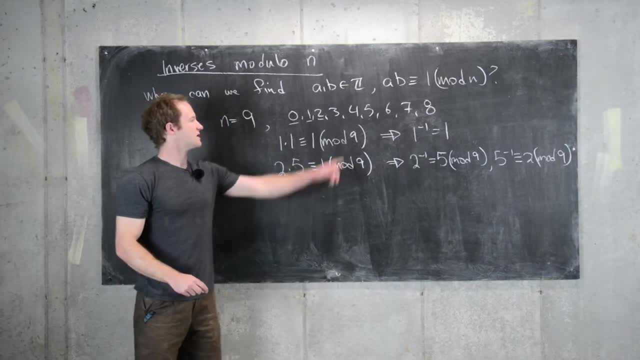 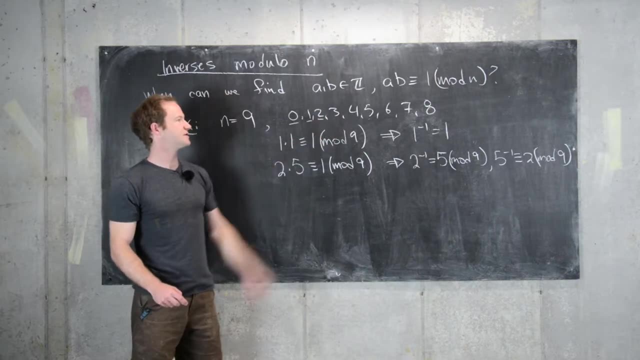 So let's look at 3.. So let's do: 3 times 0 is 0.. 3 times 1 is equal to 3.. That's not equal to 1.. 3 times 2 is equal to 6.. 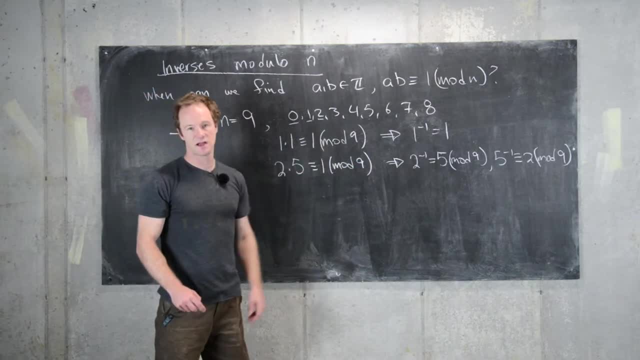 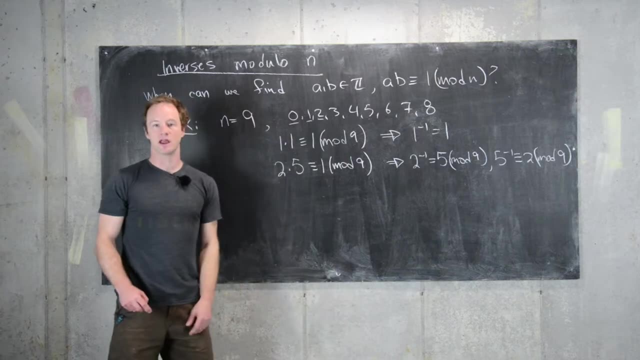 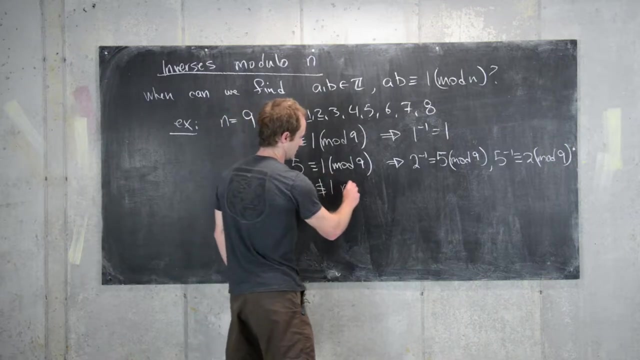 Again, that's not 1.. 3 times 3 is 9.. That's zero mod n. 3 times 4 is 12,, which is 3 mod n. And now we can keep going And what you'll notice is that 3 times x is not congruent to 1 mod n. for all x. 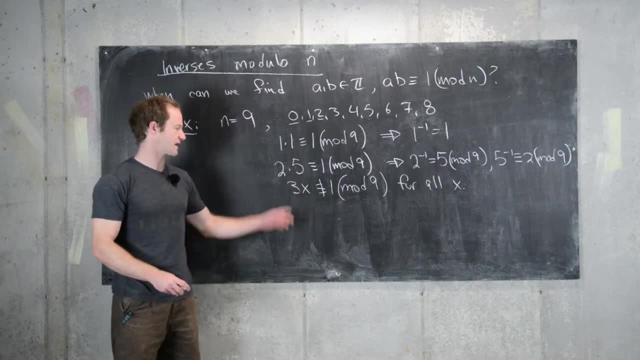 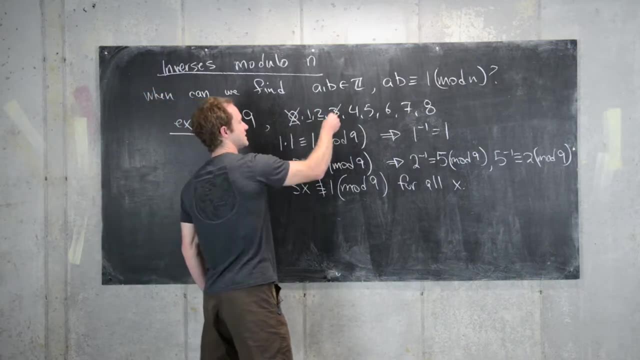 Good. So we'll prove this, why this is the case in just a second. But, needless to say, you will not have an inverse mod n. So here we have. so 0 doesn't, 3 doesn't. So let's look at. 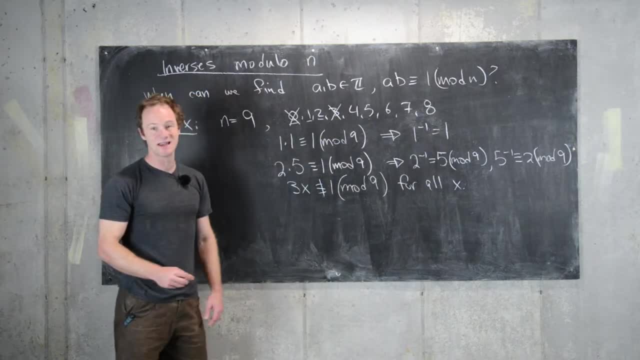 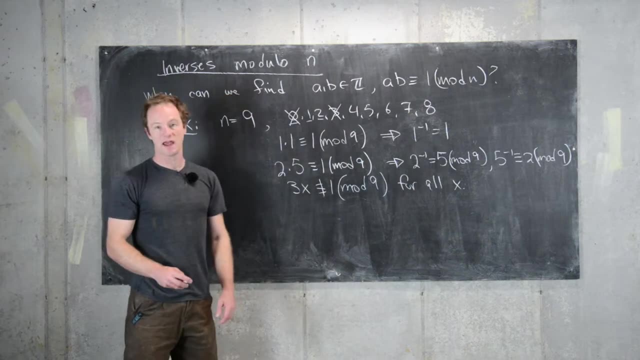 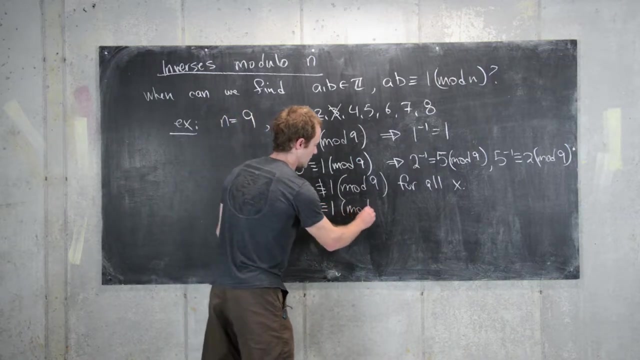 4. And so 4 times 4 is 16.. So that's not 1 mod n. But maybe let's look at: 4 times 7 is 28.. And 28 is 1 more than 27.. So here we have: 4 times 7 is congruent to 1 mod 9.. Good, And so that's. 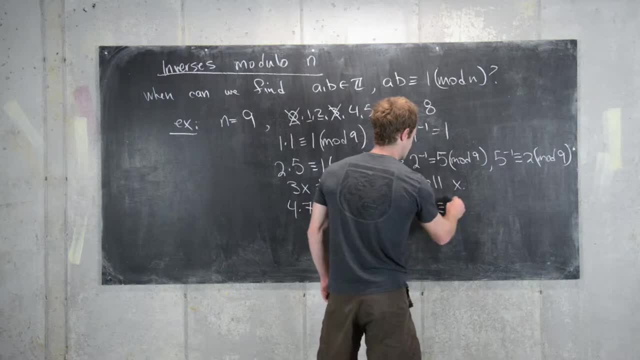 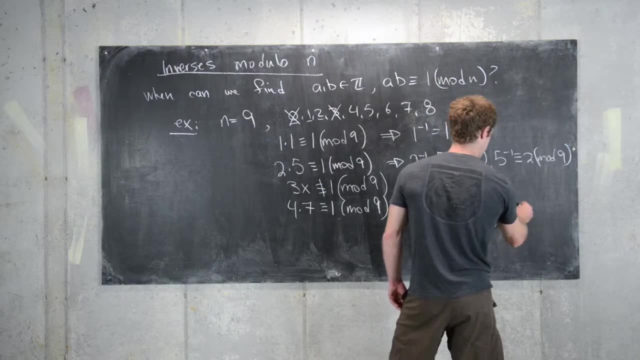 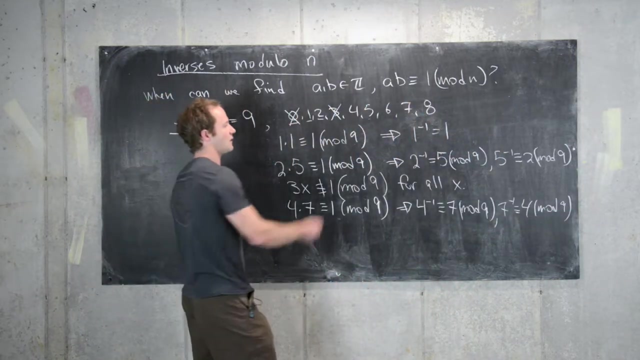 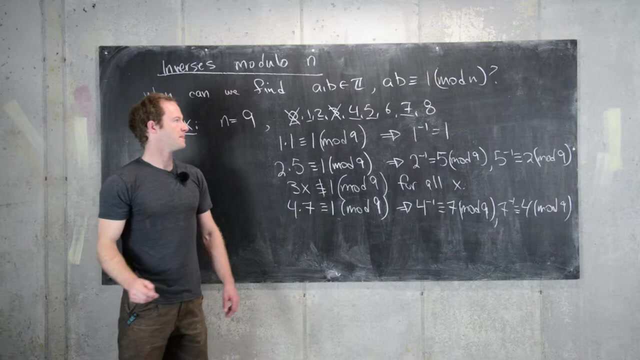 equivalent to saying that 4 inverse is 7 mod 9.. And likewise, 7 inverse is 4 mod 9.. Good, So, all at once, we've taken care of 4 and we've taken care of 7.. We've also taken care of 5 from before Now. 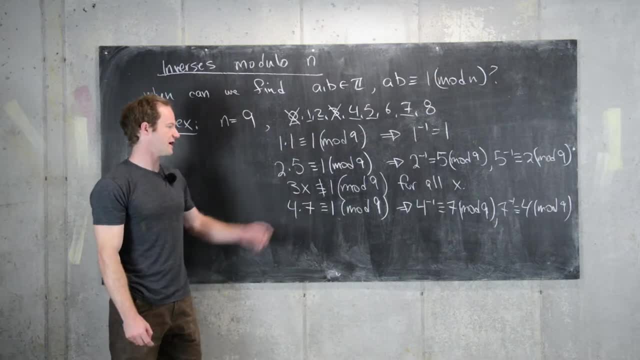 you can play around with 6 the same way that we played around with 3. And you'll notice that 4 is 1 mod 9.. And so we've taken care of 4 and we've taken care of 7.. And so we've taken care. 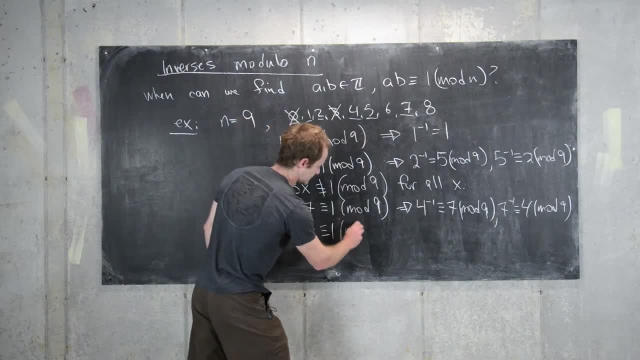 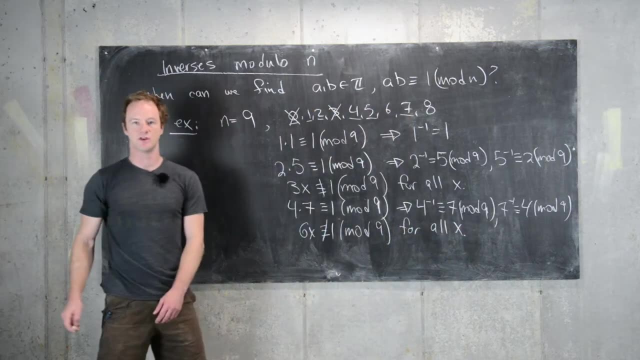 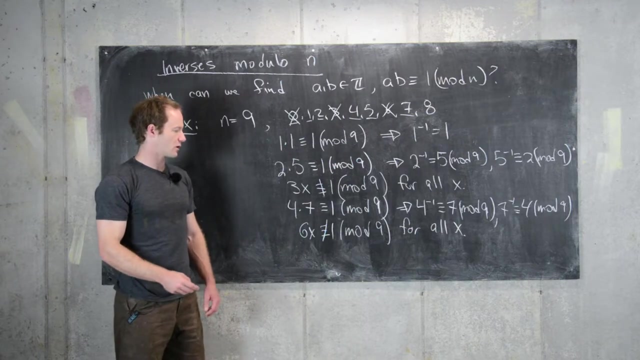 6x is not congruent to 1 mod 9 for all x. So you can't even get off the ground there. So 6 does not have an inverse. And now if we look at 8,, 8 times 8 is 64,, which is 1 more than 63. So that 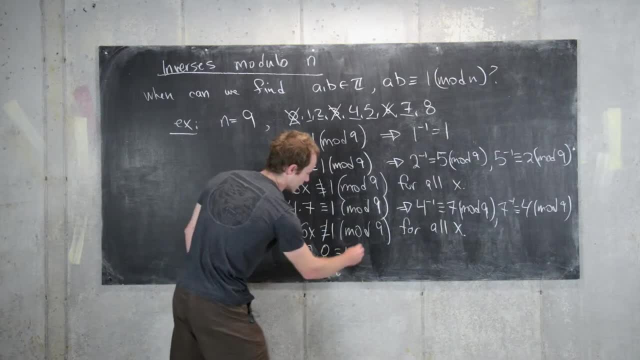 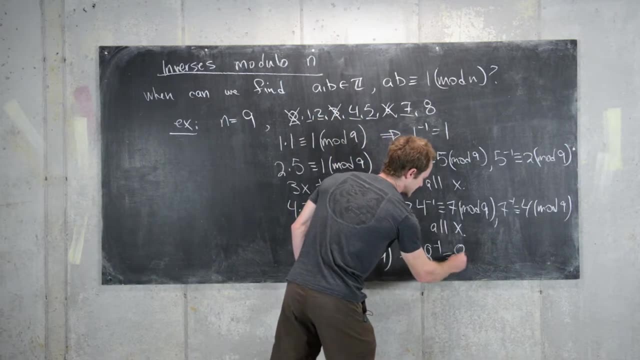 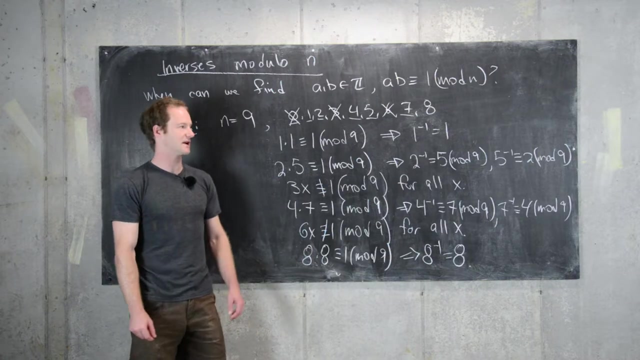 means 8 times 8 is congruent to 1 mod 9.. In other words, 8 inverse is 8.. Which makes a lot of sense, because modulo 9, 8 is equal to minus 1.. And obviously minus 1. 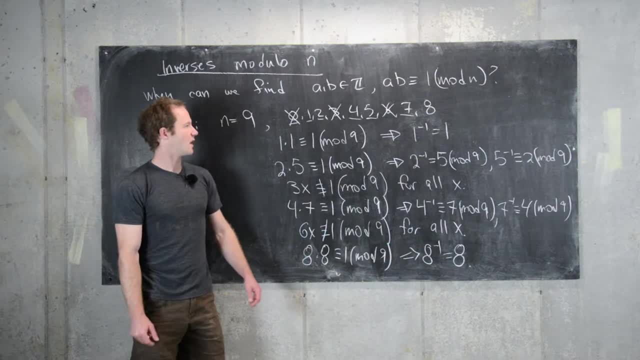 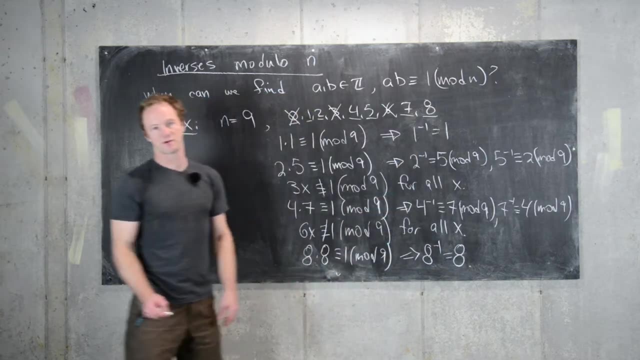 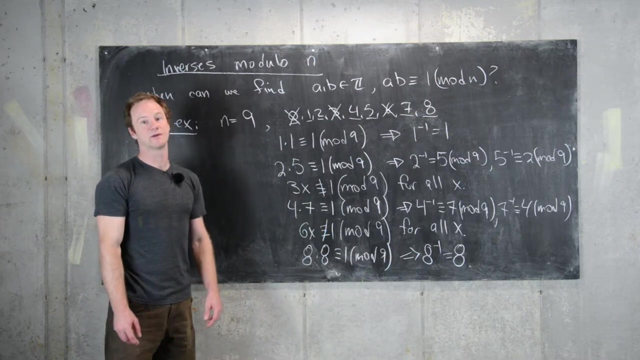 times minus 1 is 1.. Okay, great. So what we've noticed is that 1,, 2,, 4,, 5,, 7, and 8 all have inverses modulo 9.. And what is similar about them is they all are relatively primed to 9.. 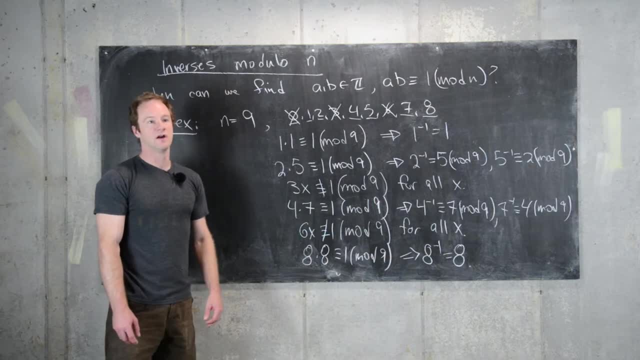 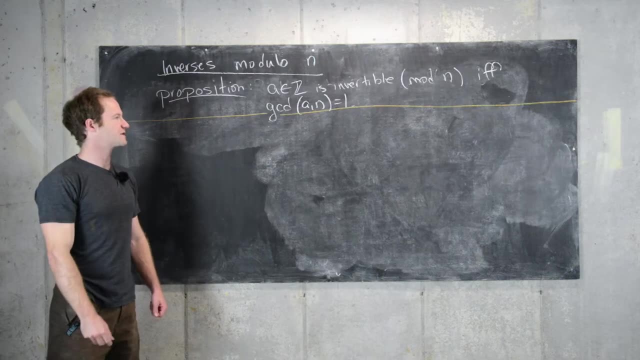 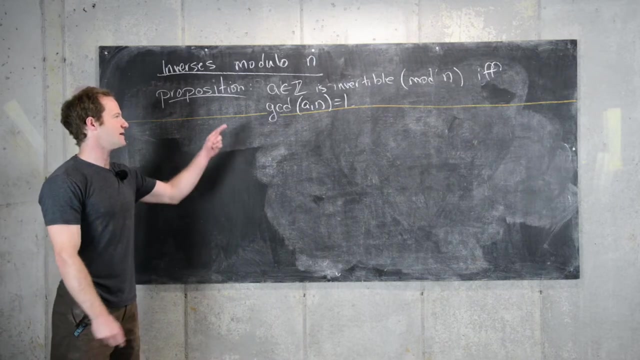 And that is in fact, the defining property of elements that are invertible modulo n. So let's clean this up and we'll prove this statement in general. Okay, so previously we gained some evidence to say that this statement should be true, So now we'll go ahead and prove this statement. So the statement is an integer a. 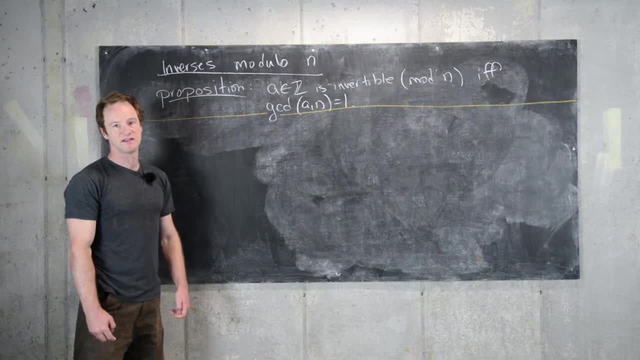 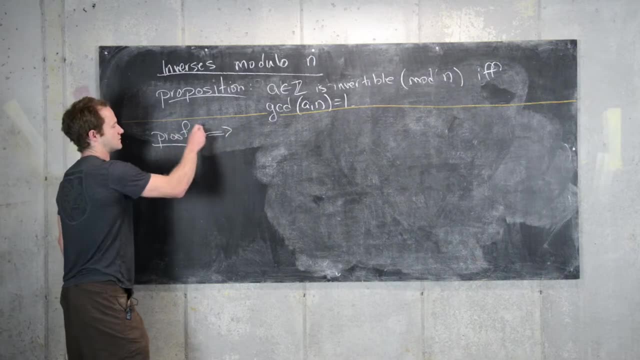 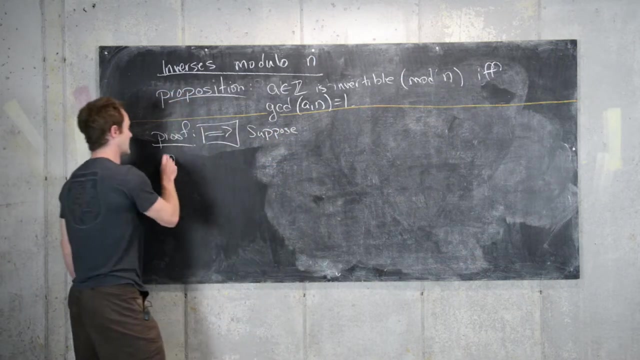 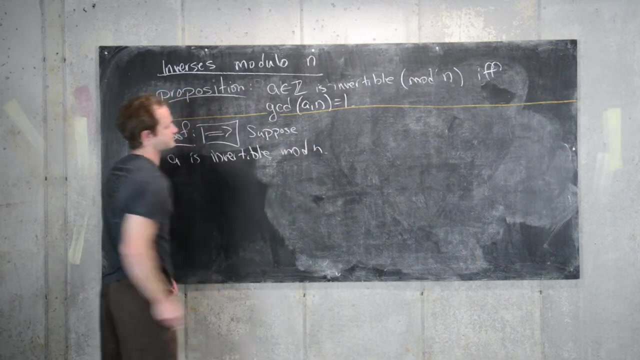 is invertible modulo n if, and only if, the GCD of a and n equals 1.. So let's look at the proof. So let's start with the forward direction. So that means we want to suppose that a is invertible mod n. So in other words, 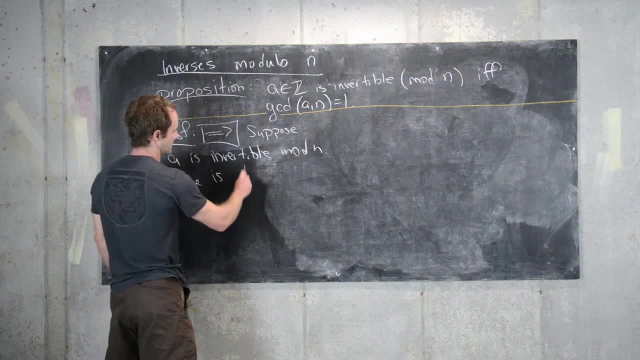 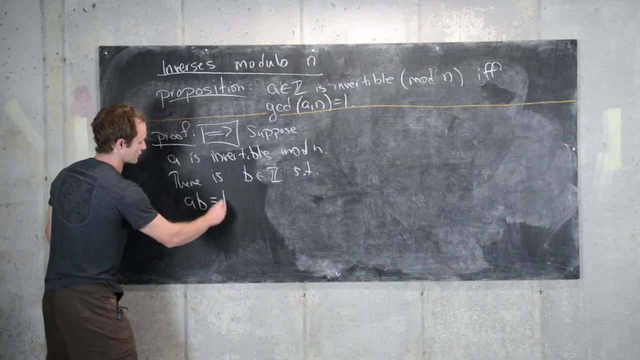 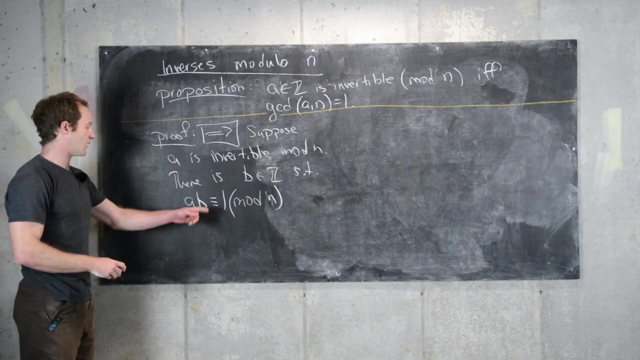 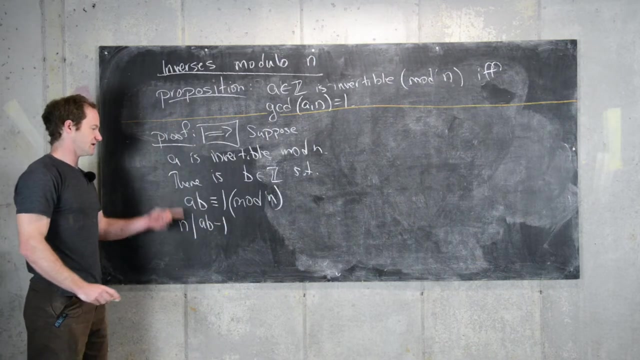 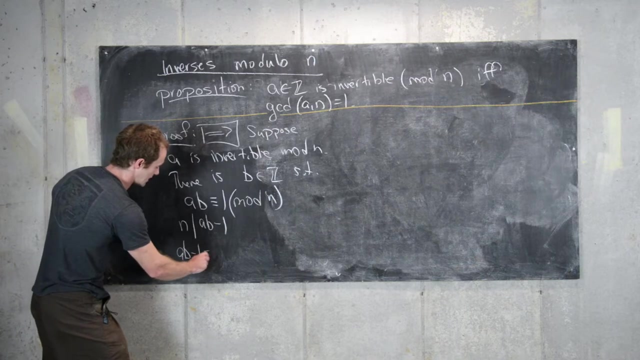 there is a b in z, such that a times b is congruent to 1 mod n. Great, Now notice that allows us to say that n divides a b minus 1.. So that's the definition of congruence: modulo n. Good, But that tells us that a b minus 1 equals n times k for some k, which is an integer. 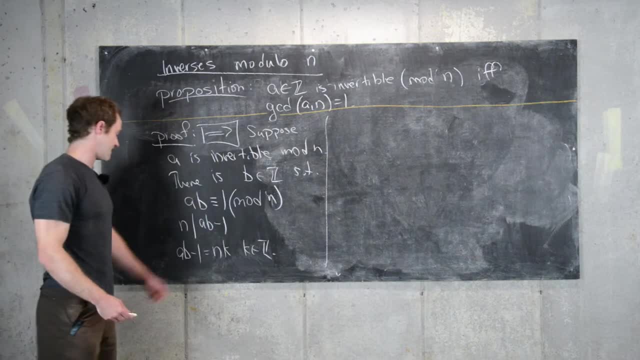 Good. And then what that tells us is that a, b minus n k is equal to 1.. So that's the definition of congruence modulo n. So that's the definition of congruence modulo n. Good, But that tells us that a, b minus 1 equals n times k. for some k, which is an integer.